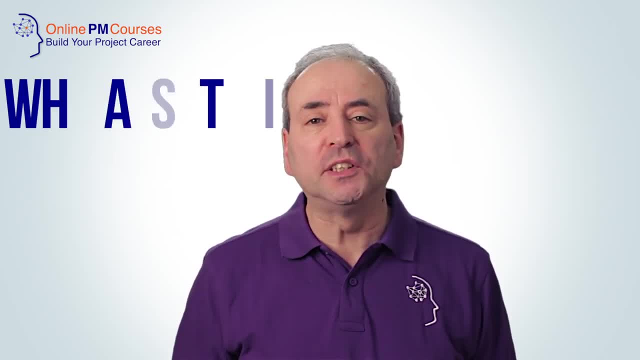 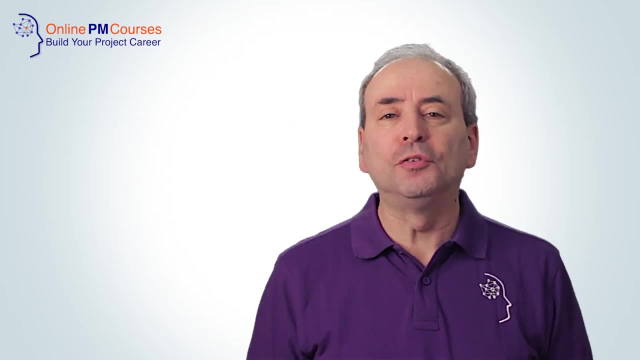 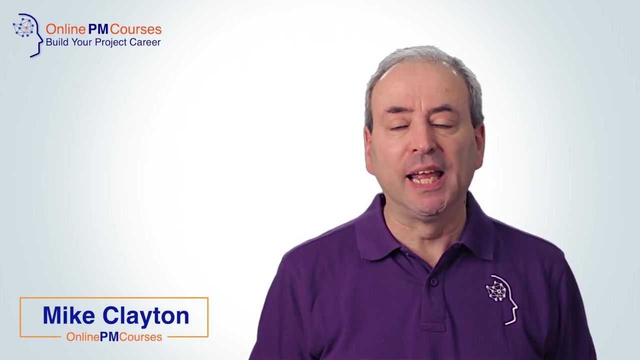 In this video, I'm going to answer the question: what is waterfall, project management? Waterfall is a specific approach to project management. In fact, it's the approach that most people think of when they think about project management. It's characterized by delivering your project in a series of stages or phases. 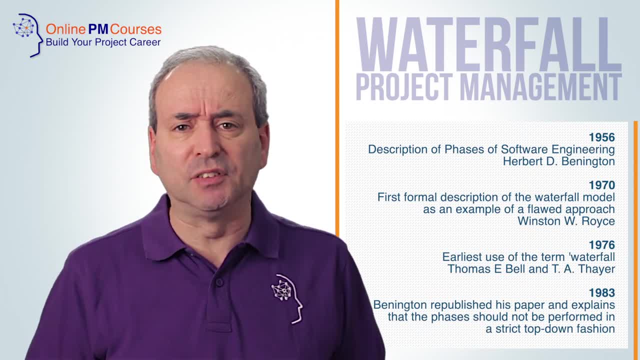 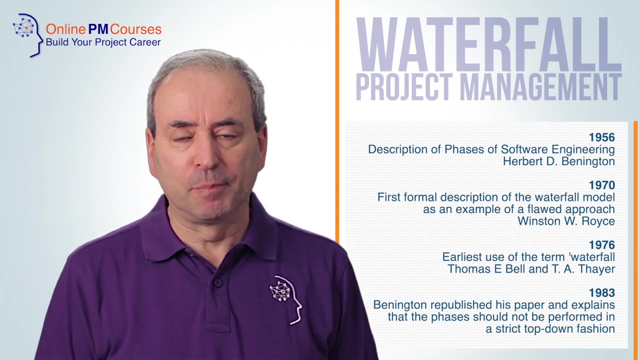 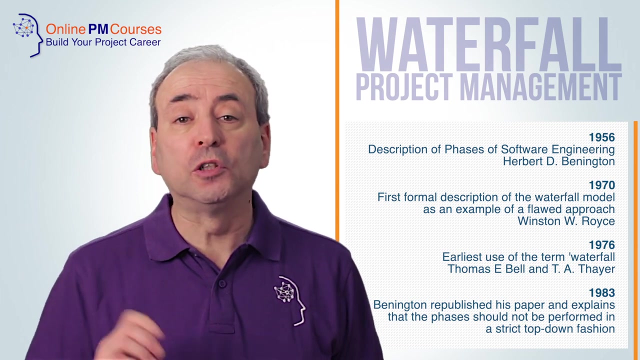 Although the term was first used in 1976, problems emerged in 1970 in an article by Winston Royce. He presented what we might call waterfall project management as a flawed approach to software development. As a result, waterfall is often used as a pejorative term in describing 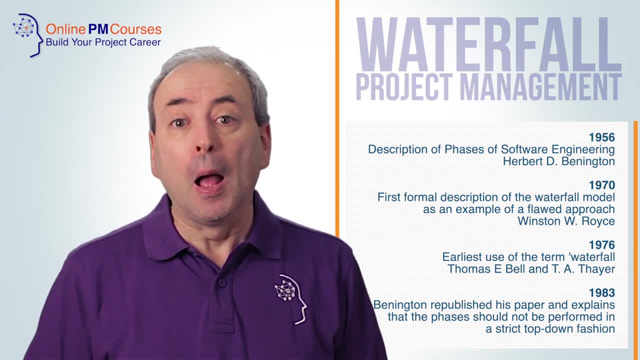 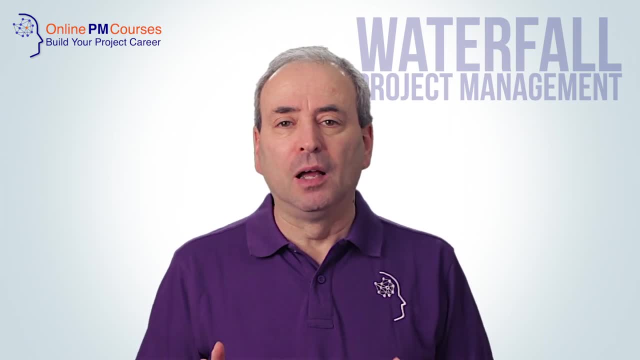 an inefficient approach to project management, But nothing could be further from the truth. Waterfall project management wasn't and shouldn't have been designed originally as an approach for software development, And the fact that it was used in the early days for software development is a sign of the immaturity of software development rather than of a weakness. 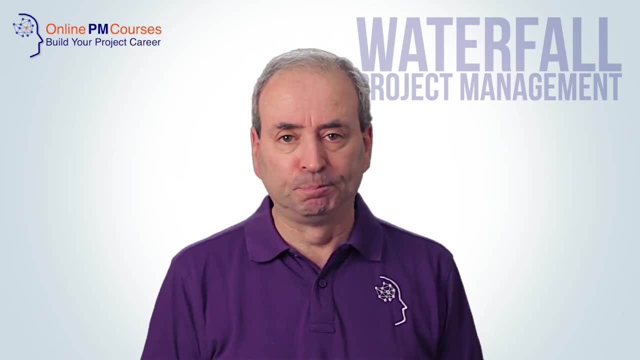 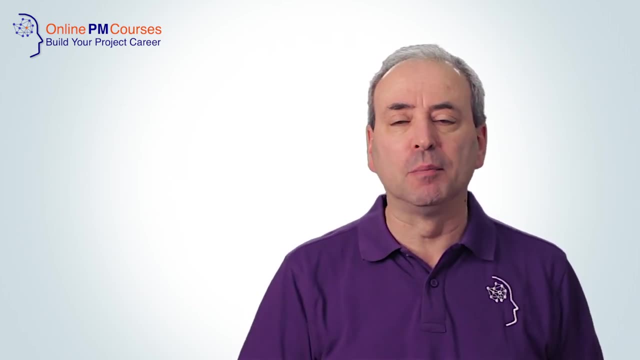 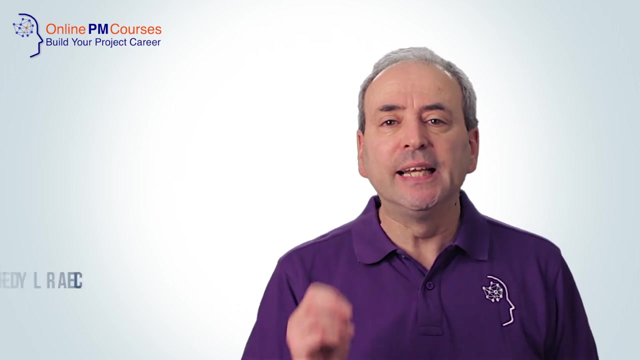 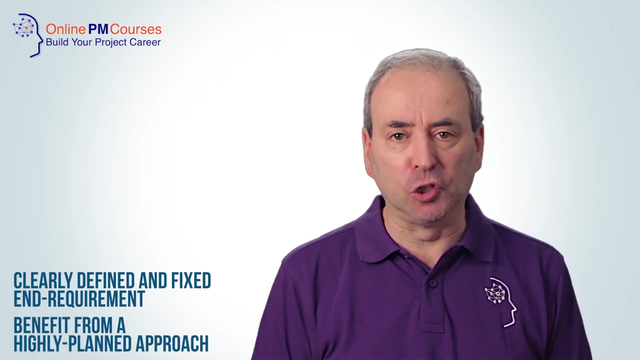 of the approach to project management in general. Waterfall project management is extremely well suited to project in other domains like manufacturing, engineering and construction. These have a clearly defined and fixed end requirement and benefit from a highly planned approach. For this reason, I far prefer the description of waterfall project management to 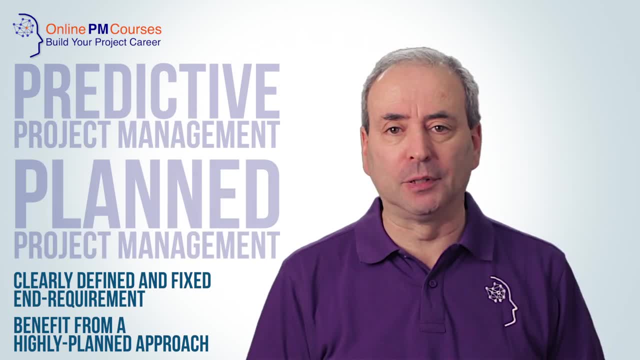 predictive project management or planned project management over the term waterfall project management, which is, after all, simply a metaphor deriving from one single diagram or representation of how it works. It also gets us away from the stigma that the term waterfall project management carries, particularly among some software development professionals and some. 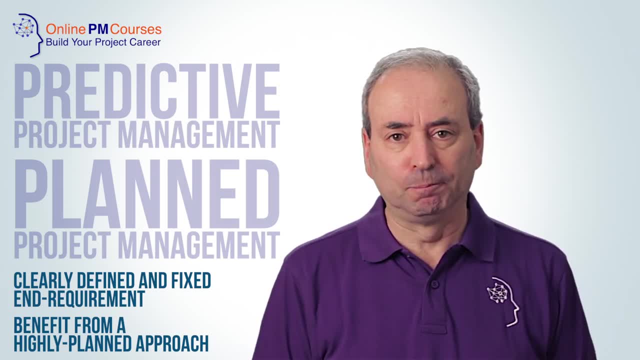 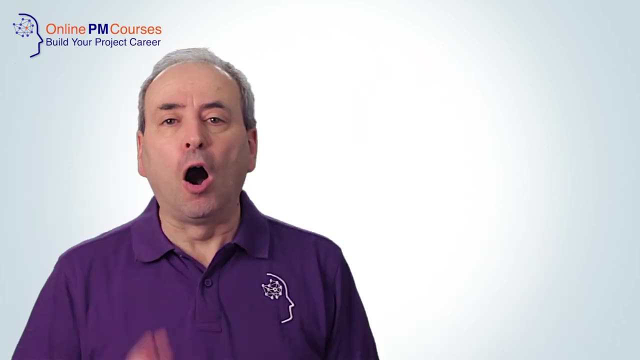 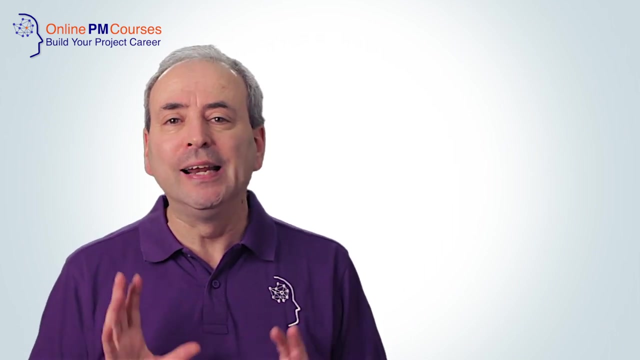 evangelical agile professionals. Yes, waterfall is poorly suited to many forms of software development, but that does not in any way negate its value as a project management methodology. Often you'll see the stages of a waterfall project represented as the stages of a linear software. 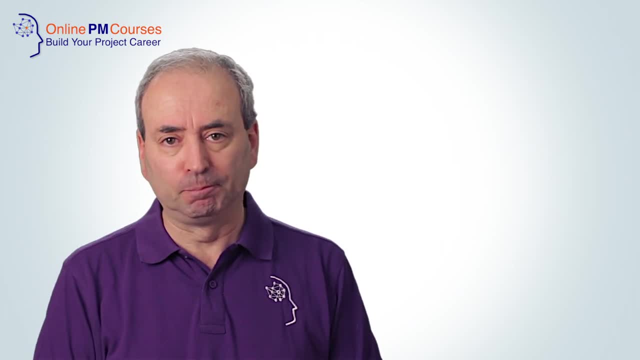 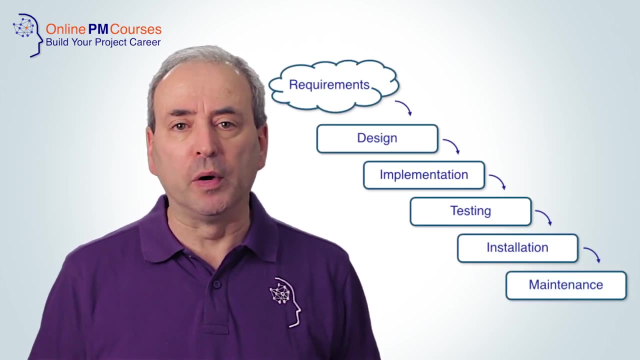 development project because of its history. A typical example of the stages you're likely to see is this six-stage model, which starts with requirements gathering, is followed by design of the solution and then implementation to create a working model. Then we've got testing to prove that model, then installation or deployment. 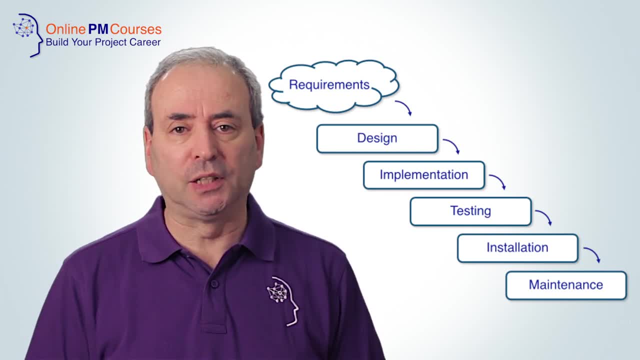 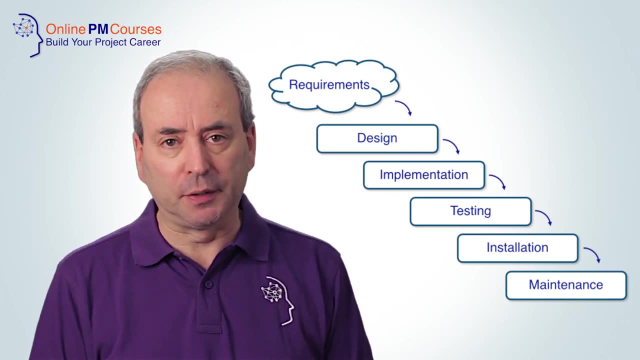 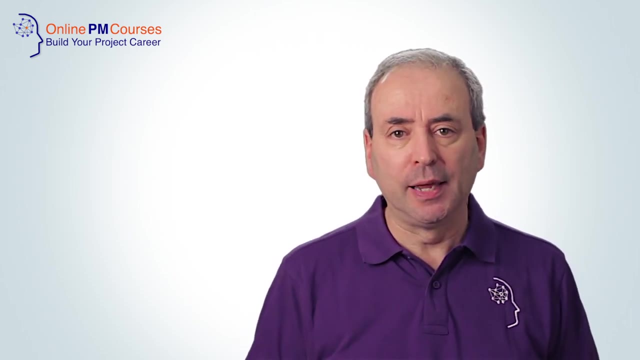 which is sometimes wrapped in with the final stage of maintenance, operation and development, In this case, the software in a live operational environment. However, I far prefer to think of waterfall, or predictive or planned project management in terms of a more generic life cycle And the life cycle that I use in all of our online PM. 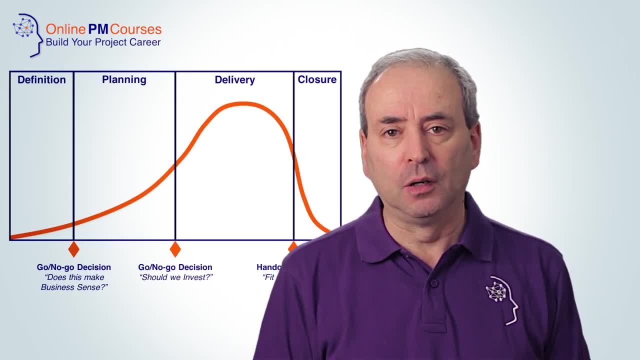 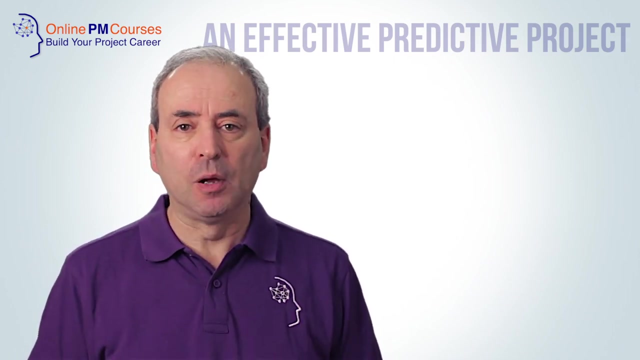 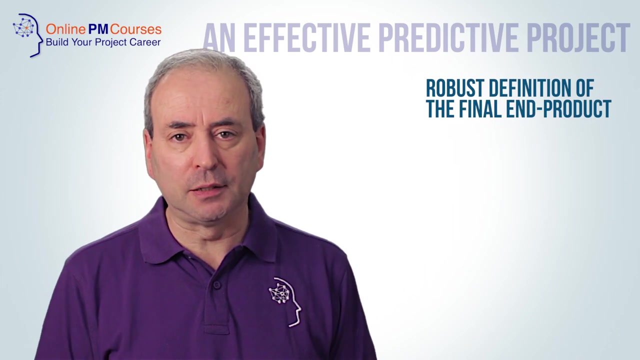 courses. training is a simple four-stage life cycle which starts with project definition, then planning, then delivery and then closure of the project, while the finished products are implemented and maintained in the operational environment. Three things typically characterize an effective predictive project. First, there is robust definition of the final end product. Secondly, careful planning. and 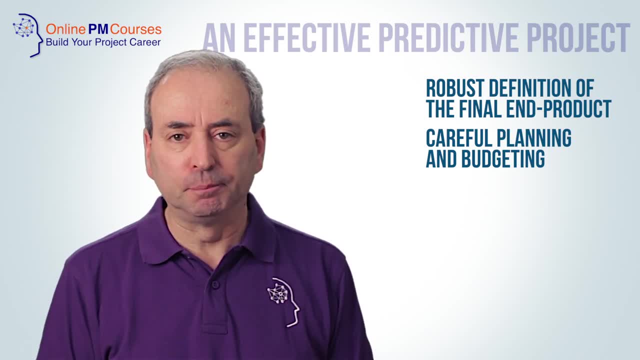 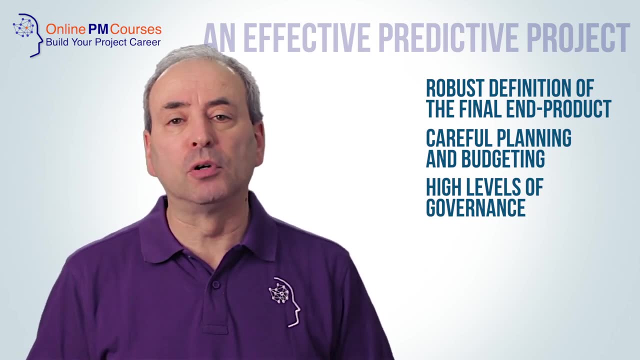 budgeting to establish how we're going to create it. And third, high levels of governance, which often means a substantial amount of project definition, which is rejected by many agile practitioners. But for the sorts of projects that predictive or waterfall project management works well in, it's got to be inevitable that we produce a lot of. 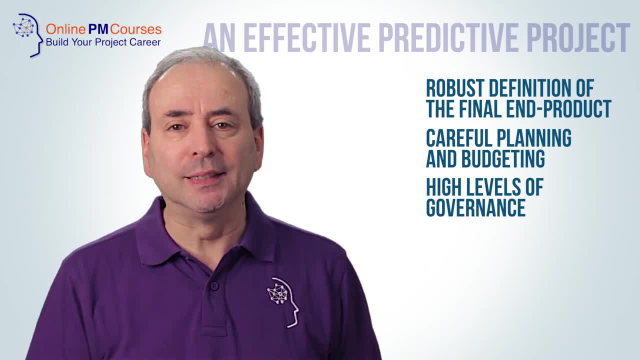 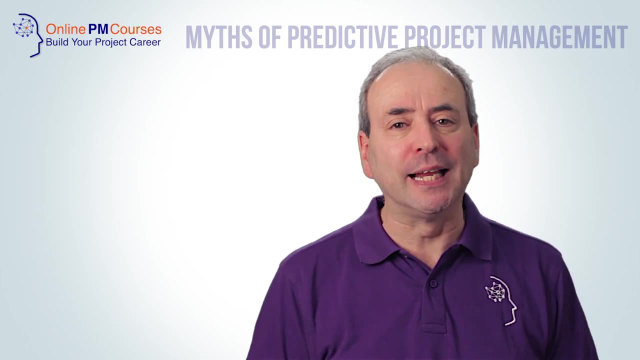 documentation, Because if you're going to maintain complex machinery or engineering, then you need people to understand how it works and the decisions that were made along the way. But waterfall, or planned project management, is often misrepresented, And there are equally three important things which are not true about waterfall projects but that are often claimed. 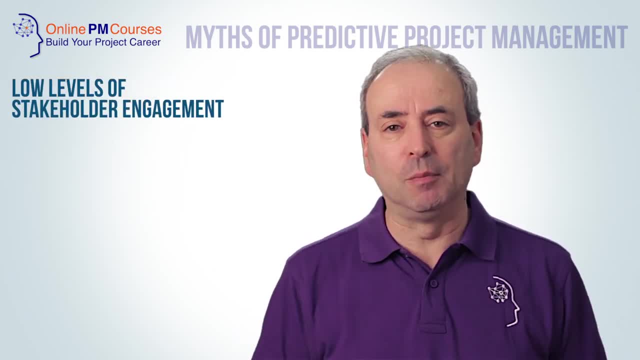 Firstly, it's claimed that they don't have sufficient engagement with stakeholders, but a well-run predictive or planned project will engage with stakeholders at the earliest stages and maintain and increase that engagement throughout the lifecycle of the project. Secondly, it is often claimed that 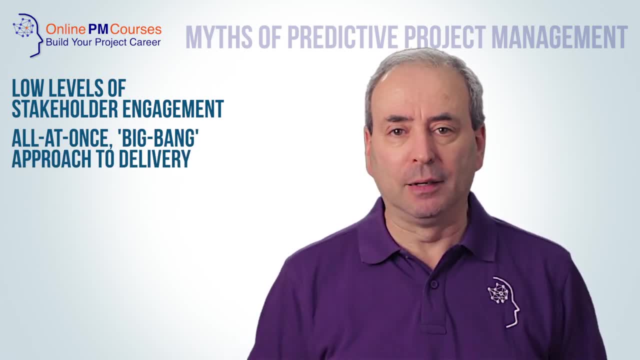 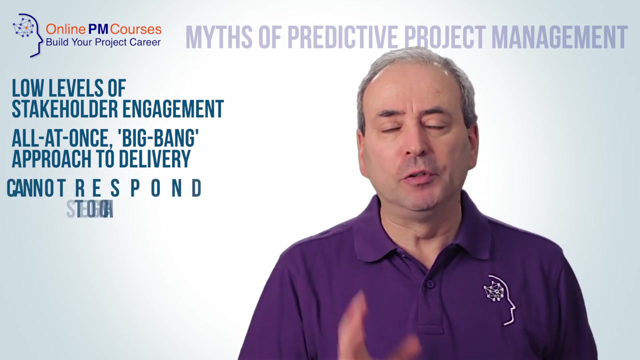 waterfall projects have an all-at-once or big bang approach to delivering the final products of the project. But again, many waterfall projects work effectively by delivering incremental benefit to their sponsoring organization. and thirdly, it is often claimed that waterfall projects cannot respond to changes. they do not. 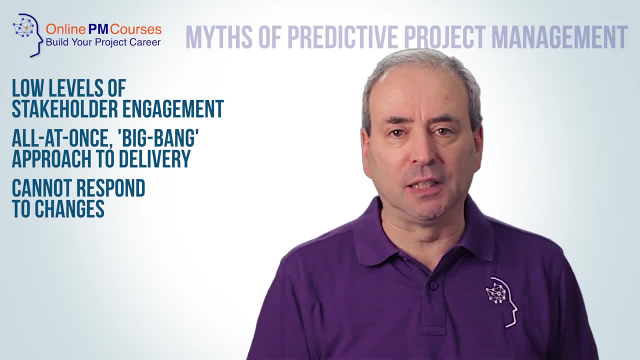 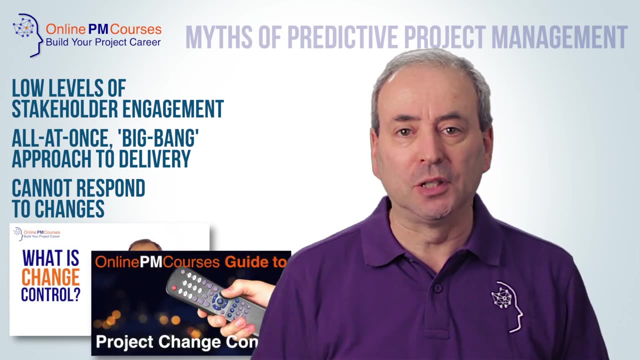 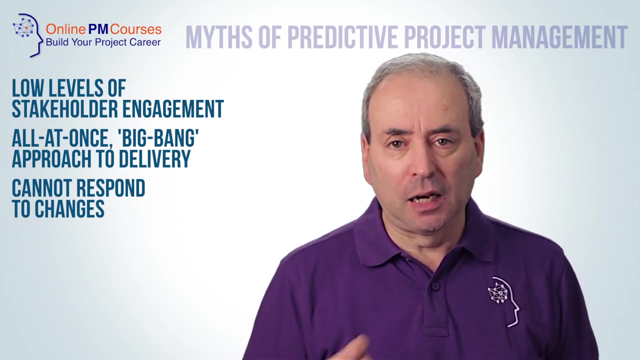 allow refinements of the original plan, the original design, the original goals and objectives. but again, in a well-run waterfall project there will be a clear change control process and i've done a video and written articles about how that works. so a waterfall project does deliver excellent client, customer, stakeholder engagement. it allows for incremental delivery of 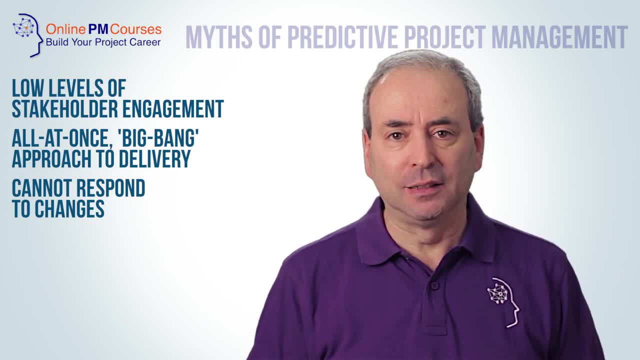 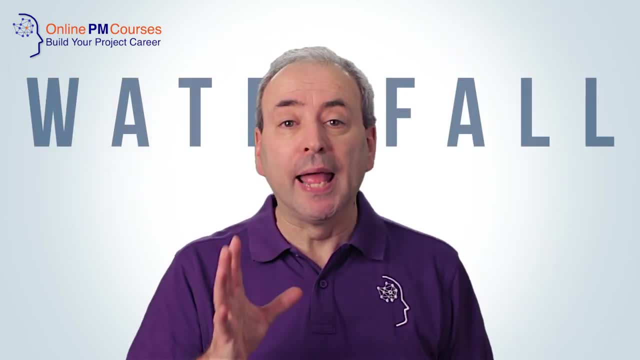 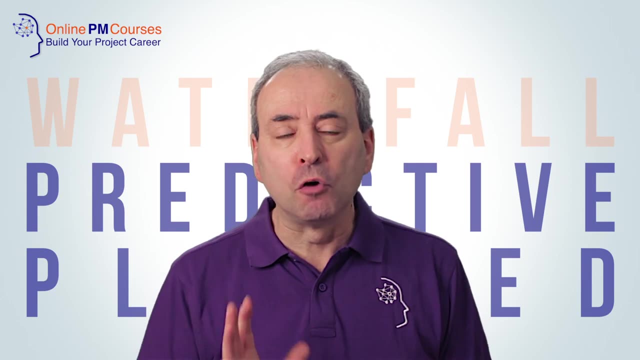 benefit and it allows for changes to specifications throughout the life cycle of the project. so waterfall project management is ill-named- best to think of it as predictive or planned project management- and for the right projects it is an excellent process and if, like me, you've learned predictive project management as your 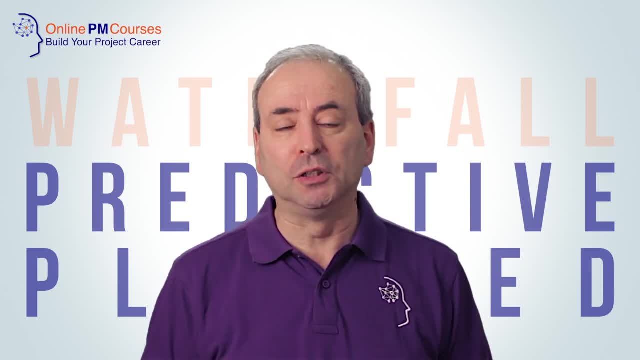 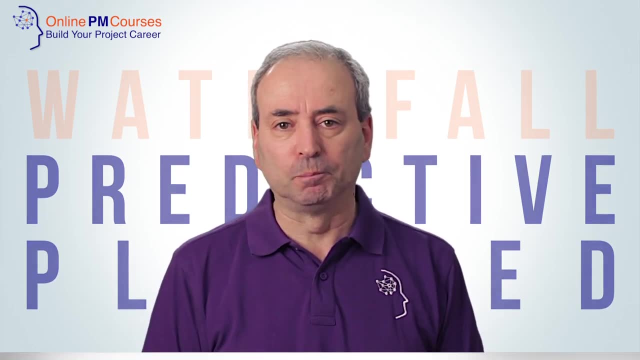 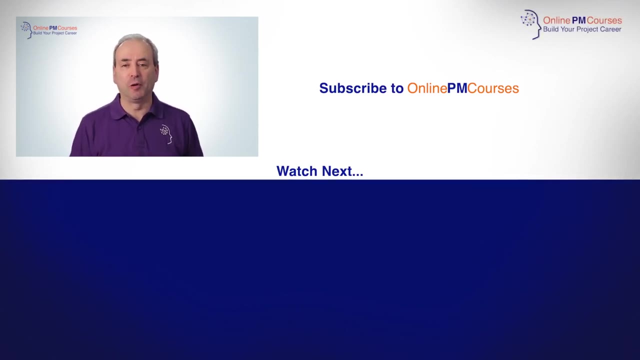 basic approach to managing projects. then be proud of what you've learned and simply recognize that it doesn't necessarily apply in every circumstance. please do give us a thumbs up if you like this video. i'll be creating loads more great projects for you in the future. 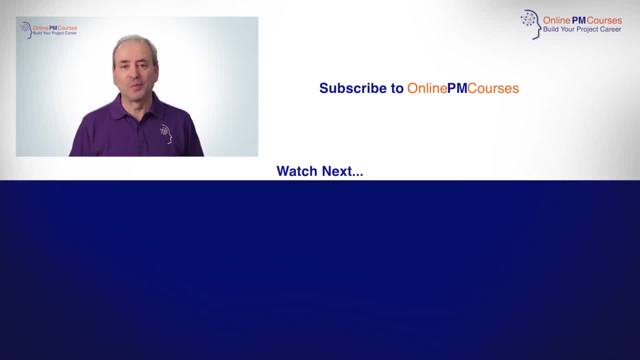 project management content. so please subscribe to our channel and hit the bell so you don't miss any of it, and i'll look forward to seeing you in the next video.